summation, we incur a round of error And we add other numbers And in floating-point arithmetic. every time we do a summation we incur a round of error. So we start with one number, we add other numbers and in floating-point arithmetic. every time we do a summation we incur a round of error. 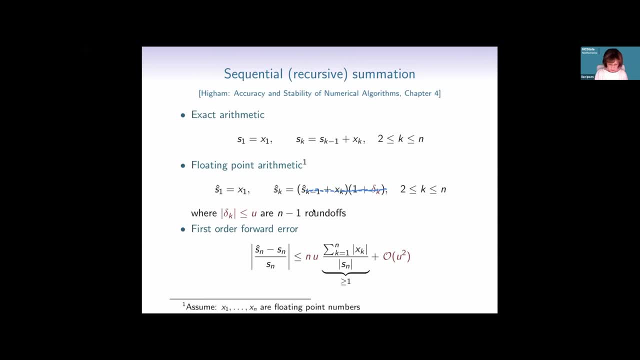 Now, every summation involves all the previous quantities, And so of course, it's x1 and x2 that get subjected to the most round-offs. since we do n additions, We have n-1 round-offs, and then we get this bound here, Partly the n coming from. 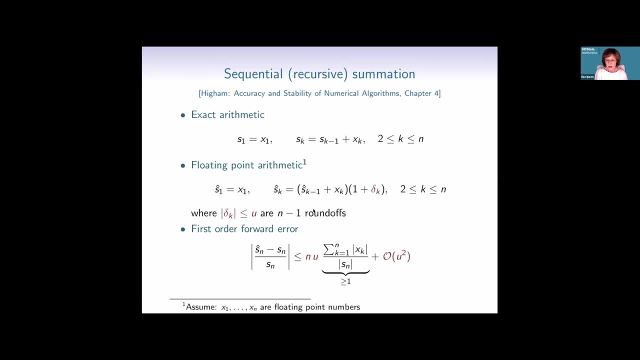 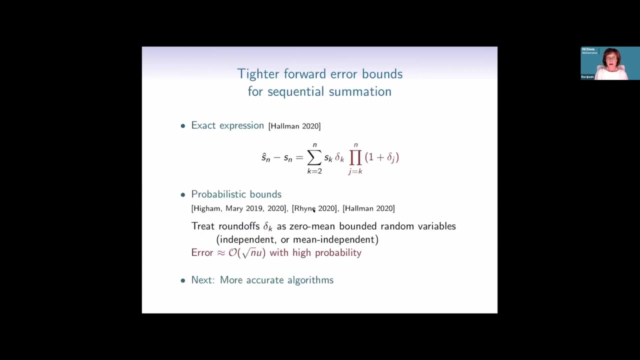 x1 and x2 being subjected to basically n round-offs, And we see a condition number here, and that says that if all the summands have the same sign, the problem is well conditioned. If they don't have the same sign, we may have cancellation in the denominator here. Okay, so we 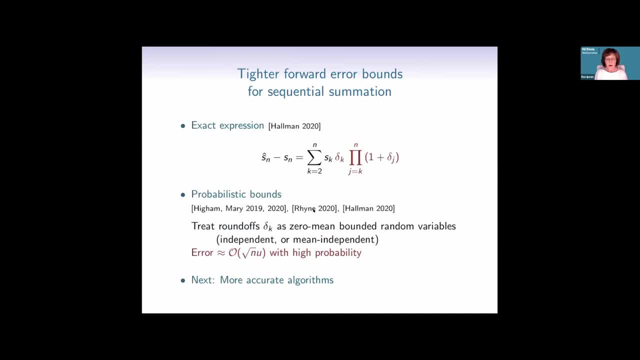 could have tighter error bounds and there has been quite a bit of effort lately. So Eric has just an explicit expression for the error in sequential summation and nothing big. but I'll come to it. I'll come back to it later, that's why I'm putting it up. Then there are probabilistic bounds, so, Nick, 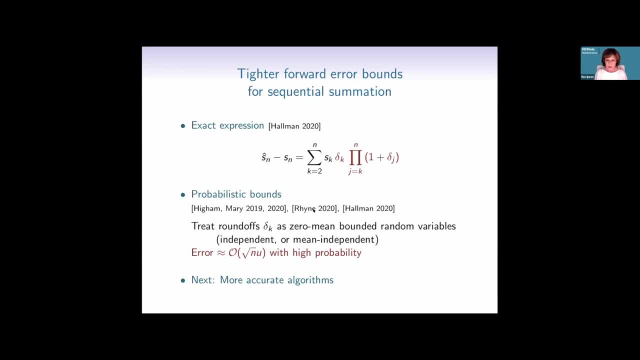 has been involved in that, Where one treats the round-offs as random variables bounded zero mean and they can be independent or mean independent, And then with high probability one can show that the error is proportional to a square root of n times the machine precision rather than n times the machine. 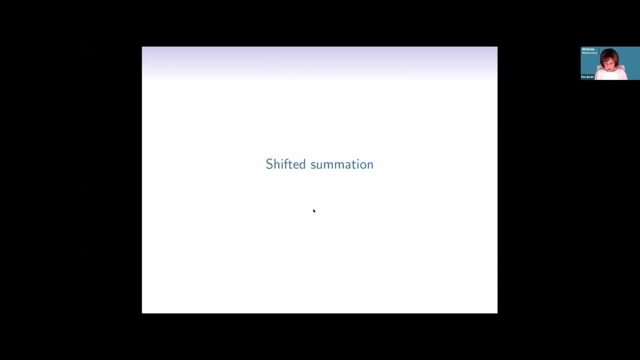 precision, And now we are wondering how can we come up with more accurate algorithms. So he has shifted summation, which is really motivated by what people doing, computer architecture and formal methods for programming. So that's a good example of what we can do. And then we have the other. 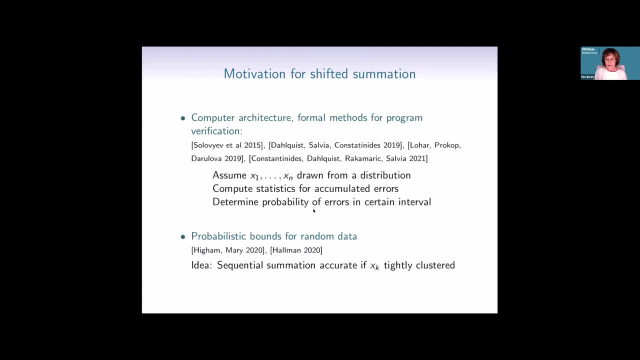 program verification, where they try to automatically verify the correctness of a program. So they assume that the inputs are drawn from some distribution. then they go compute statistics for the accumulated errors and then determine the probability that the accumulated error is in a certain interval. Now that is. 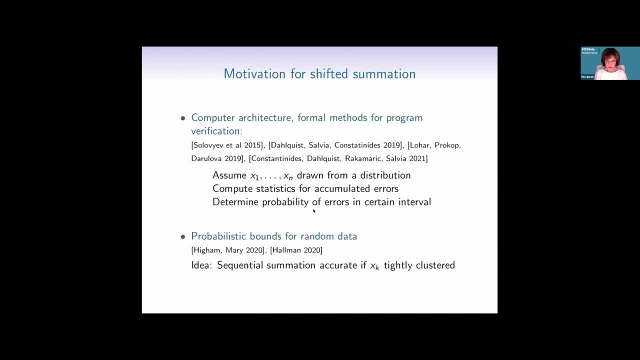 really awkward, unwieldy and not very feasible. So then, prompted by this, Nick and his collaborators look at probabilistic bounds. probabilistic bounds for random data, And the idea here is that sequential summation is accurate if all the summons are tightly clustered. So here is. 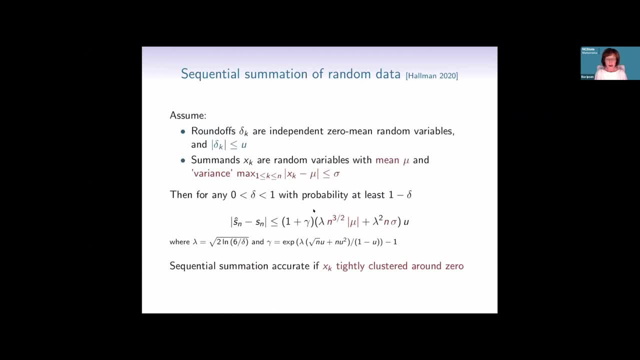 the bound, that Eric improved upon what Nick and Teo had done. So assume the round offs are independent, zero mean, random variables of course, bounded by the machine unit round off, And let's assume, let's assume our summons are clustered around the mean. 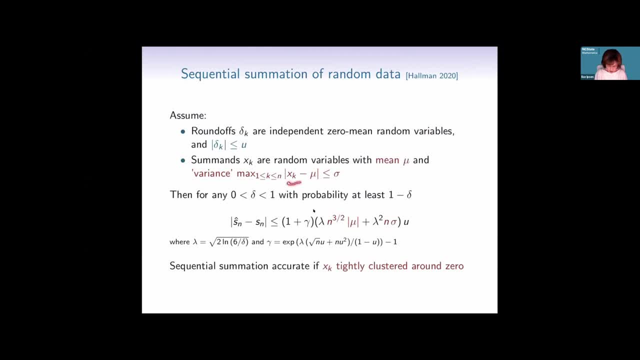 and have a variance. this is a variance in apostrophes. this is just the distance from the mean of all the summons that's bounded by sigma. then one can show with high probability that the forward arrow is bounded about by this expression. Here we have the 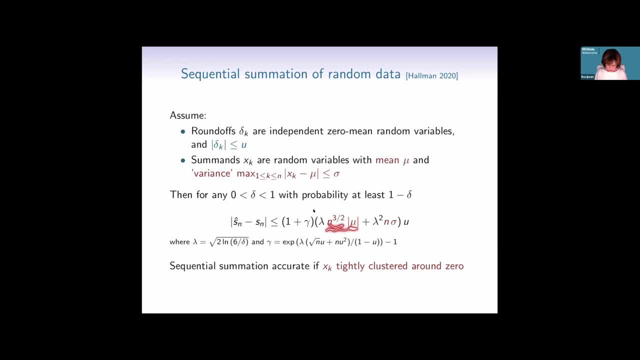 mean. if the mean is small or close to zero, then this thing is small. Here we have the variance that the difference from the mean. well, if the summons are tightly clustered, then this thing is zero. So the qualitative conclusion here is that if, if you have random data that are tightly 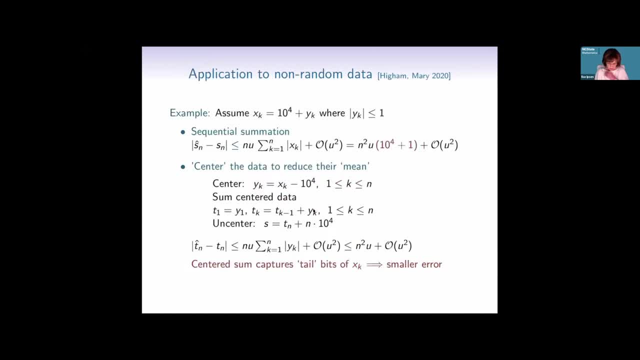 clustered around zero, your error should be much smaller. So then, Nick and Teo went on to apply this to non random data. So here's an example. Assume all our summons are 10,000 plus a number that's less than or equal to one. So if we do sequential 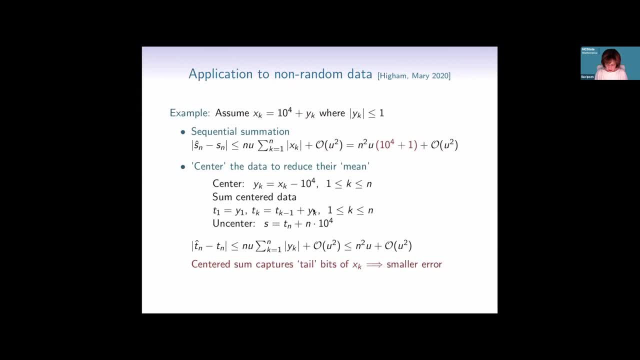 summation and look at the first order: error bound. well, everybody is in magnitude, at most 10 to the four plus one. However, instead, the idea that Nick and Teo had is: let's center the data. So, basically, this: what this does is it removes the most significant. 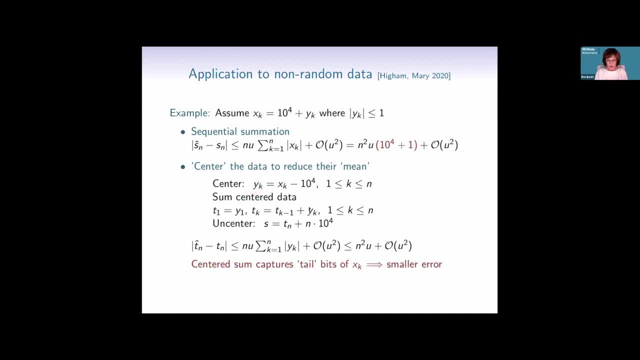 bits so that the y k retains the tail bits or the least significant bits. then we compute the sum from the least significant bits And then at the end why, you know, all the 10 to the fourth that we had subtracted we have to add back. 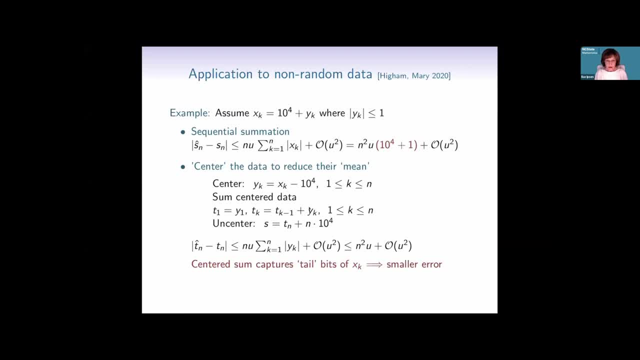 But the idea here is to do that for non random data is a little like compensated sum Summation: the centered sums capture the tail bits, the least significant bits of the summons, and therefore we incur a smaller error. So here's a shifted sequential summation algorithm. 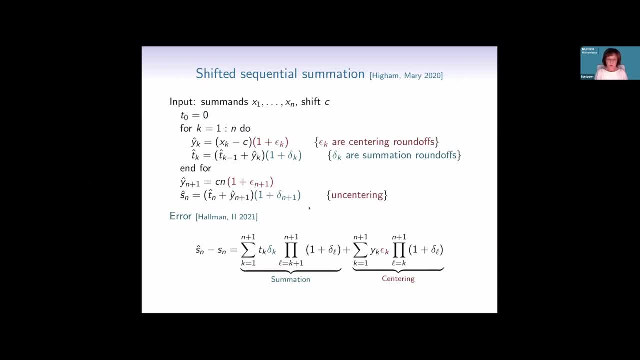 that Nick and Teo have in their paper, And we have two types of round of errors here. We have the round of errors, the red ones we incur from centering, And we have the blue ones that we incur of Yeah and the blue ones that we just incur from. 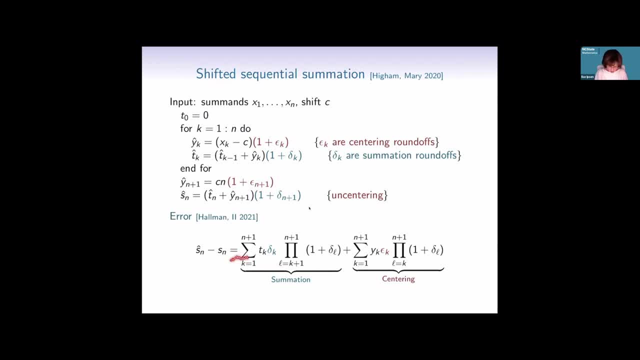 summing up, And then we can show explicit expression for the arrows. that comes in two neat parts. The first one is basically the error that we would get from summing up, And the second part is the error that we incur due to centering. Now, if we could do. 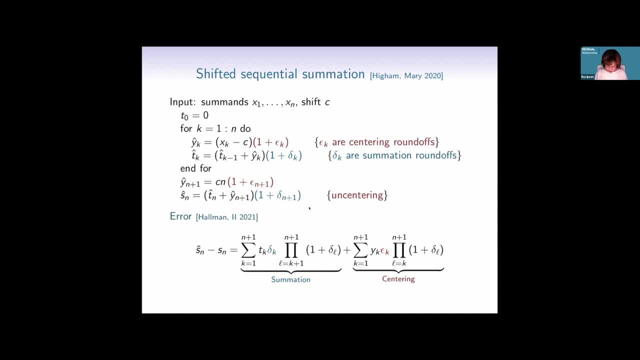 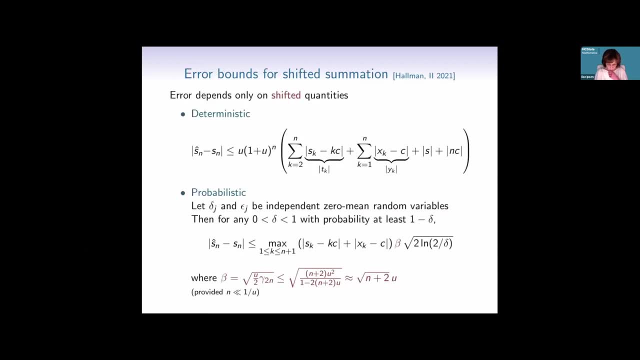 the centering exactly accurately. then this thing would go away and we get just the expression that we got for sequential summation. Okay, so this is all well and fine, but we need bounds. So this previous expression gives an error. bound, that is phrased just. 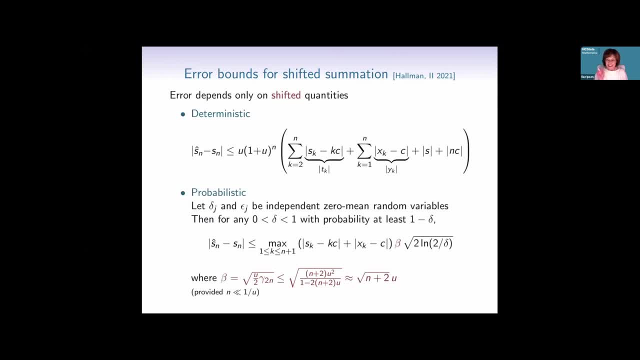 in terms of the shifted quantities, in terms of the exact shifted quantity. So I guess it's called a priori bound And then if we, then we can also provide a probabilistic bound. So again we assume our all our round of errors are conveniently. 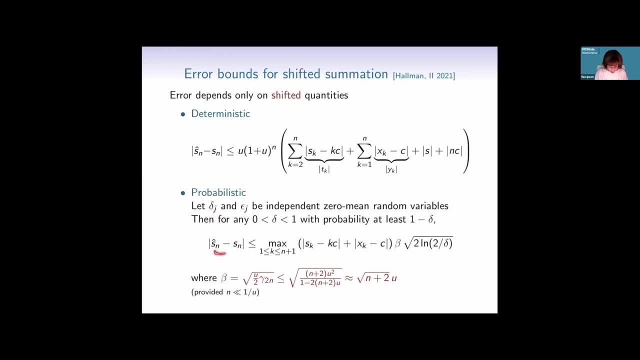 independent zero mean random variables. then we have a forward arrow that's bounded in terms of a maximum. that is basically the maximum intermediate partial sum times beta, and beta is- I can't use my my pen here because I'm running out of real estate- beta is basically square root of n times unit round. 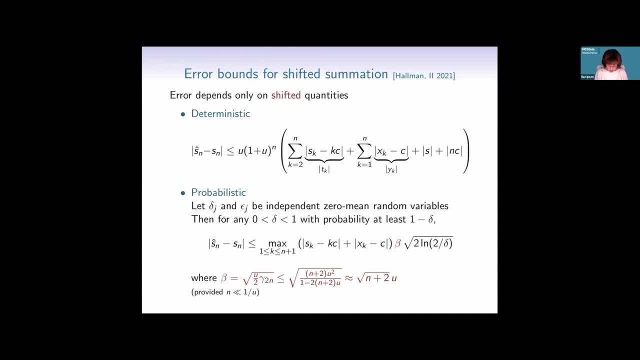 of then. this is a small factor. So, and this is the, the maximum shifted sum is basically what Nick says, section 4.2 in his book. I always remember his book of section four, everything that to minimize that the partial sums, is the way to make a summation. 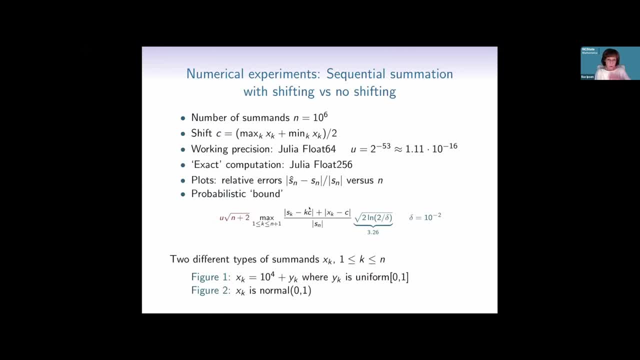 more accurate. So let's look at some numerical toy experiments. So we have 10 to the 600,000 summons we use as the shift, the largest plus the smallest over two. So it's an approximation to the empirical mean. the working precision here is 64 bits in Julia and the exact 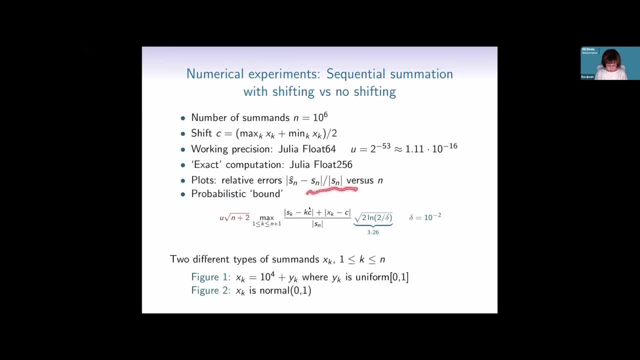 computation is 256 bits. we plot the relative errors and then the probabilistic bound. it's not quite the bound. I just took this factor And then we're going to look at two different types of summons: the tightly centered summons, around 10, 10,000.. And 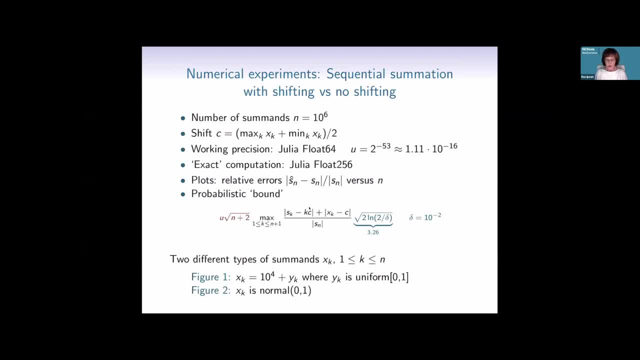 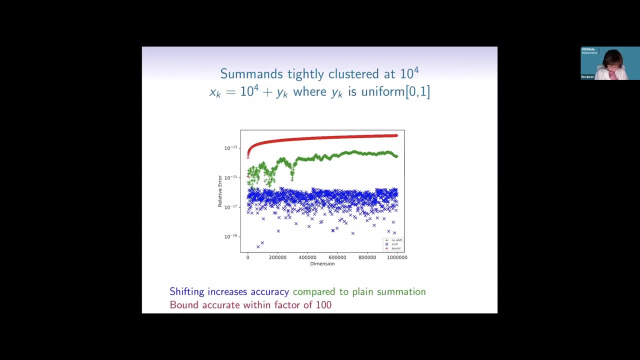 then summons that are normal 01.. So normal, standard Gaussians with the mean zero and variance one. So what we have here? we have the problem size. on the horizontal axis we have between 10 to the 19 to 10 to the minus 13.. On the vertical axis, blue is shifted. 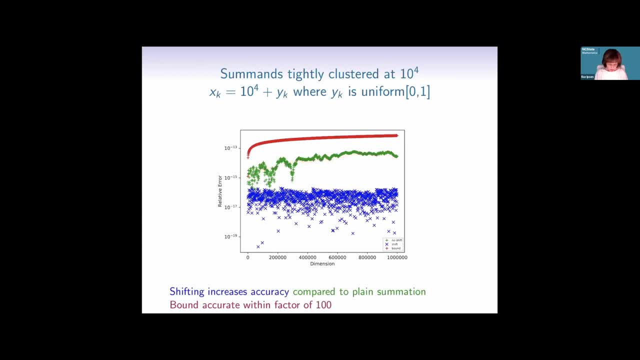 summation: Green is plain summation And this is our bound. So when the summons are tightly clustered, that shows that shifted summation can be more accurate by by a factor of 10 or 100 and plain summation And our bound is qualitatively good. 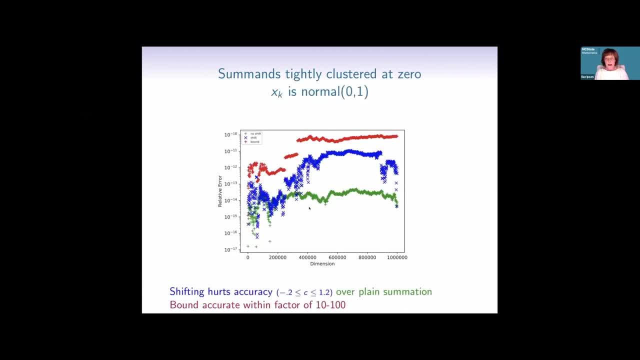 and within a factor of 100.. However, if you take summons that are tightly clustered at zero- and this is not necessarily while condition problem, because we can incur cancellation- So then you see, here is 10 to the minus 1710 to the minus 10.. And you see that. 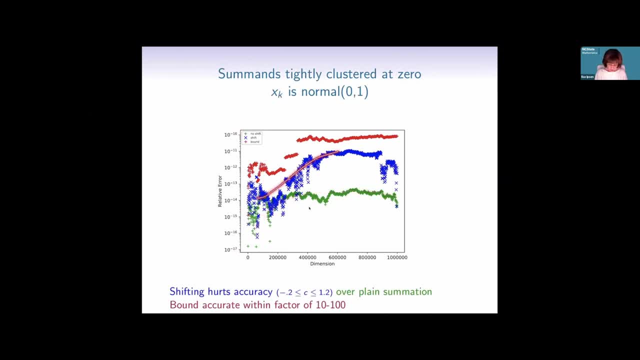 plain summation actually is more accurate than the shifted summation. And here's our bound, our probabilistic bound. So again, the bound is within a factor of 10 or 100.. But this time shifted summation actually is does damage to the accuracy. So our summary: 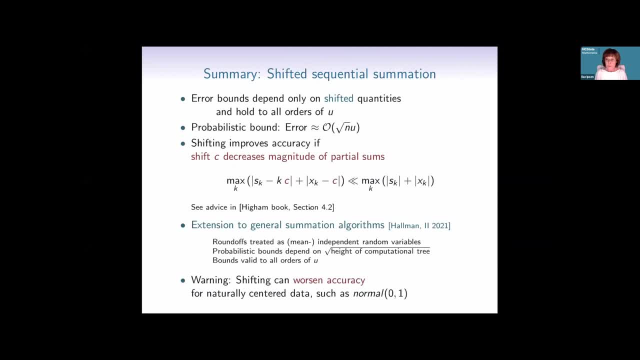 here is that the arrow bounds we have depend only on the shifted exact quantities. they hold to all orders, the exact bounds and the arrow is proportional to square root of the number of summons rather than number of summons, And shifting improves the accuracy. If the shift decreases the 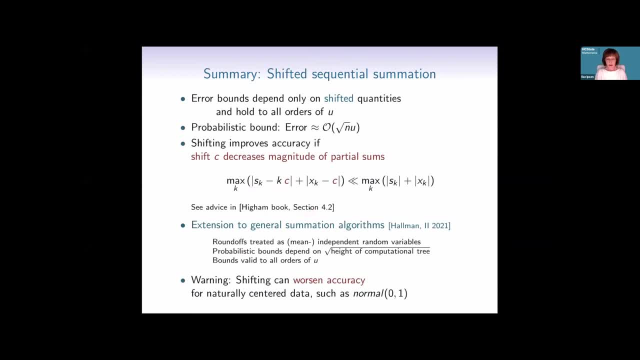 magnitude of the partial sums- exactly the advice that Nick gave in his book. So we have extension to general summation algorithms where we treat the roundoffs either as mean independent or independent. random variables and probabilistic bounds depend on the square root of the height of the. 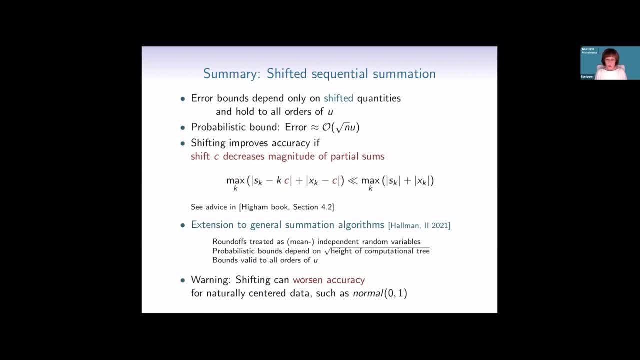 computational tree. Again, the bounds are valid to all orders. So the warning is that shifting can shifting can worsen accuracy, especially if one has data that are naturally, naturally centered. Okay, so let's go on to Kahane's method now. 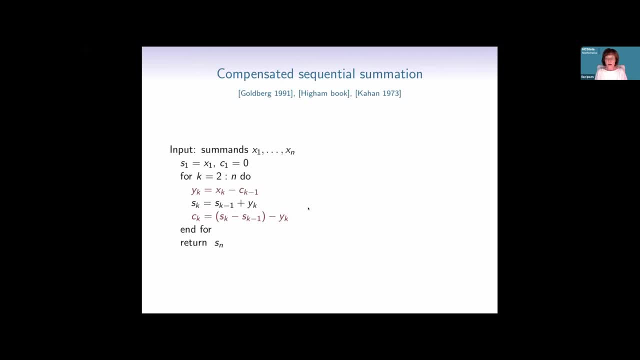 So this is compensated. sequential summation. So Kahane had a one page paper in 73. And here's his method. Okay, so what happens is we add things. these are the partial sums, we these are our summons. After we've added the next summons, we recover the. 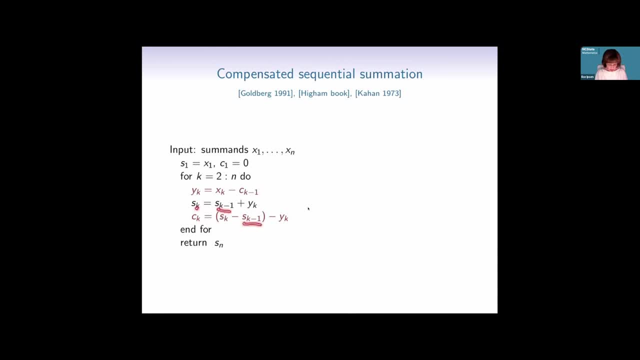 arrow in the summation. So this is the partial sum. we subtract this and this, So this is supposed to recover the arrow in the least significant bits. Then we take this, infuse it into the next summons and hope that thereby we decrease the arrow in the whole sum. Okay so, 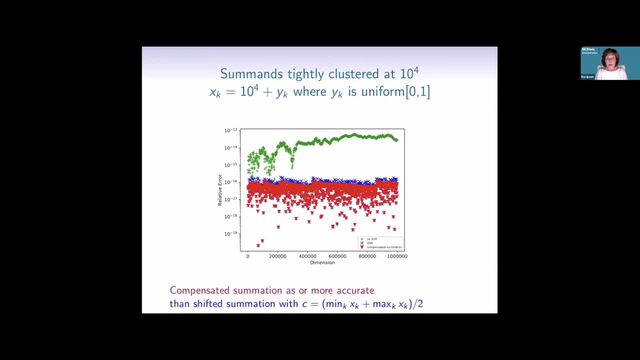 let's just compare this with centered summation. So again we have tightly clustered summons at 10,000. And we add a little bit with a uniform or zero, random variable And then you see, here is 10 to the minus 1910, to the minus 13,. we are plotting. 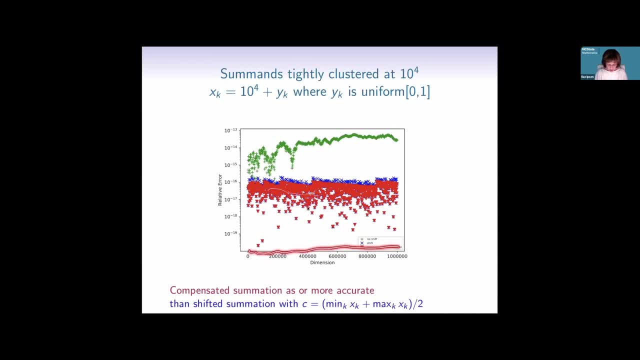 relative errors against the number of summons. Red is compensated summation, blue is centering and green is plain summation. So we see that compensated summation is at least as accurate as centered summation. If we have not a problem, that's not necessarily well conditioned where shifting. 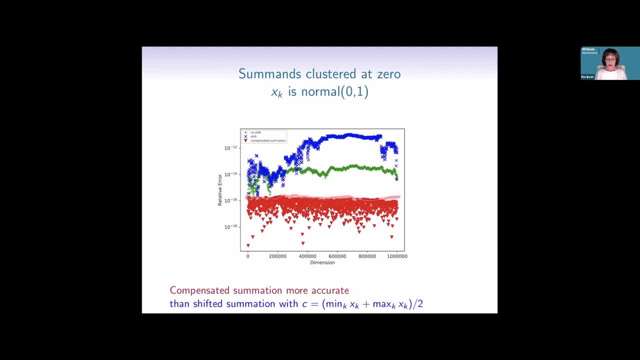 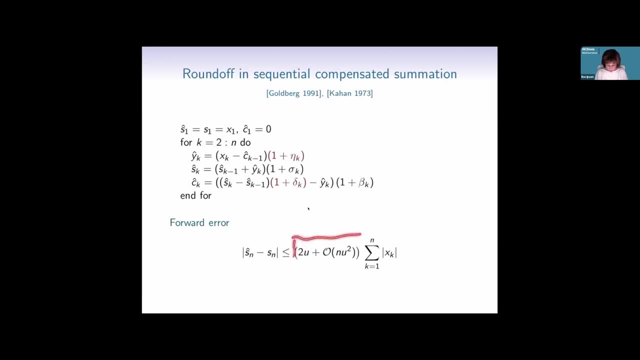 can actually do damage. we still see that compensated summation gives us machine precision, accuracy. Okay, so now we went on. So now you can see- Oh, but we know, we know about for for compensated summation summation, Why we wanted to just explore that a little further. So in 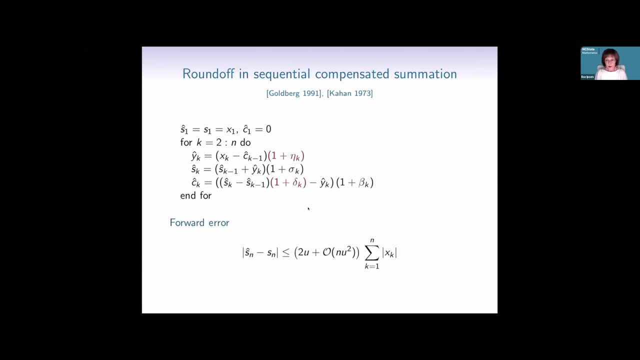 compensated summation. you're doing three more additions, so it's going to be more expensive. But we have round of errors for each additional addition that we do, And the red ones here are associated with the with the correction. then the traditional forward arrow bonus says that the error is only into first. 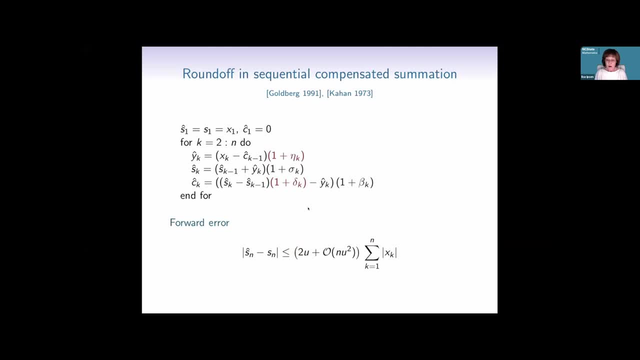 order two times you, independent of the number of some summons. we, we order, we add up plus n u square. Okay, Off we go And we derive a couple of explicit expressions for compensated summation. we get the expression for the forward arrow and for the correction And we do a little vector. 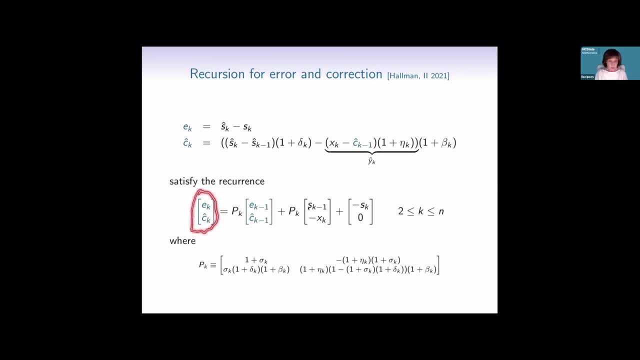 recurrence where this. these are the. this is the error and the correction. when we form the partial, the kth partial sum, it's related to the previous partial sum By matrix PK. that has only the round of errors of the kth addition in it and then some sort of stationary terms. So 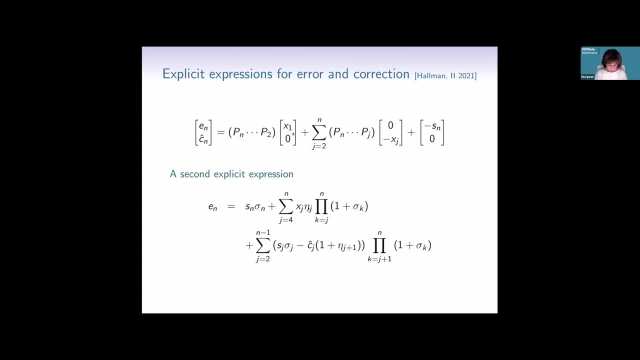 with that, we can get an explicit expression that depends only on exact quantities, not computed quantities. Okay, we have a second expression just showing off. This is not so great because it involves computed quantities And further more. we have a third expression, And this now makes it easy to. 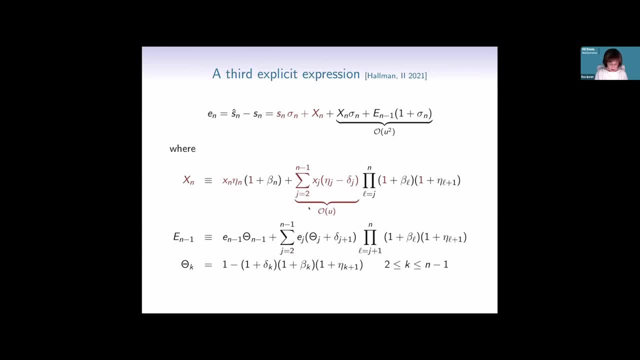 read off the local the first order errors. So this is the error and the computed sum minus the true sum it's equal to the error. we get in the last summation a lot of second order stuff plus this here. this is you can see first order error. So you can read off the. 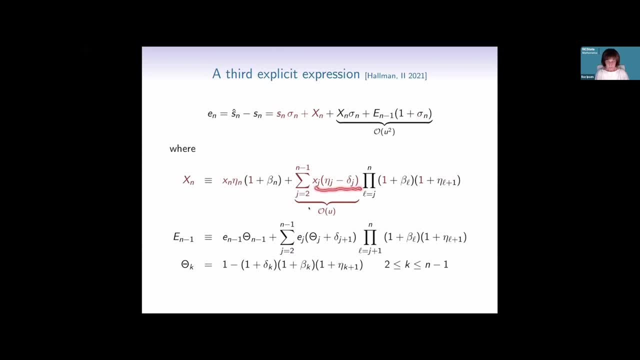 first order errors this and then these guys. So with this we can get a bound, So an expression to to, to, to second order. So the error then is the, the round of error we get in the final summation, the round of errors we get in the. 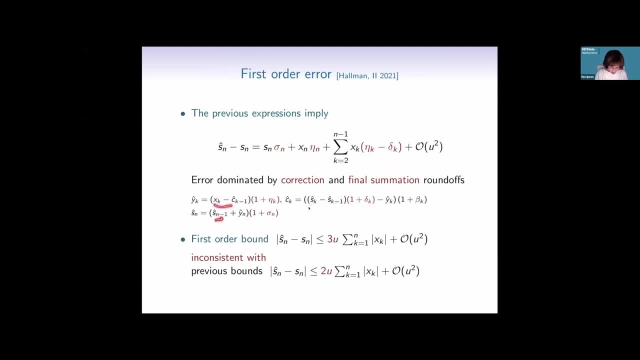 correction steps, So we can actually identify particular round of errors and everybody else. So here you can count errors 123.. So our bound then is three u times the usual sum, And that is not income. it's inconsistent with previous bounds which say to you: 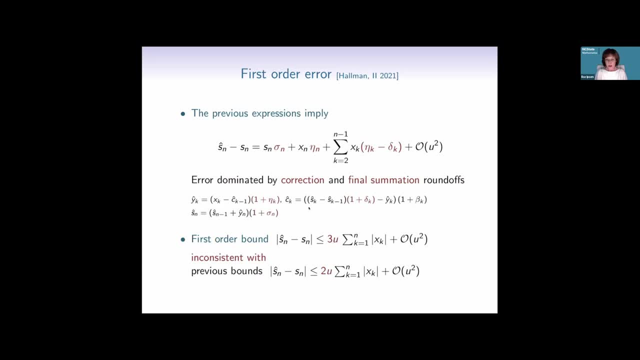 And that's why we would derive three explicit expressions, actually independently- Eric derived something, I derived something, and independently we came to the same result, And I think it's because Goldberg, in his analysis, looks only at x1 and x1 is afflicted by one less round of error than all the other. 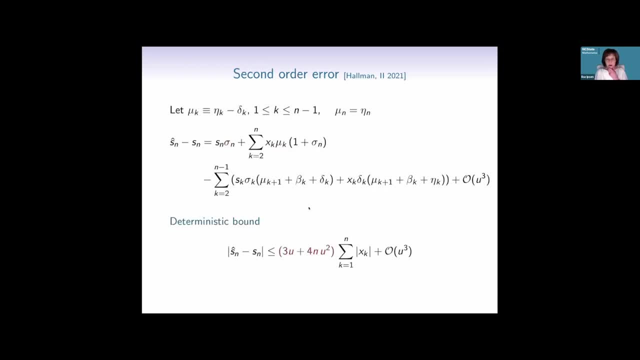 x's. So I think that may be the reason. So we can also get a second error bound, a second order error bound. You don't need to look at this, But when you actually look at the deterministic bound you have three times machine unit round off and then 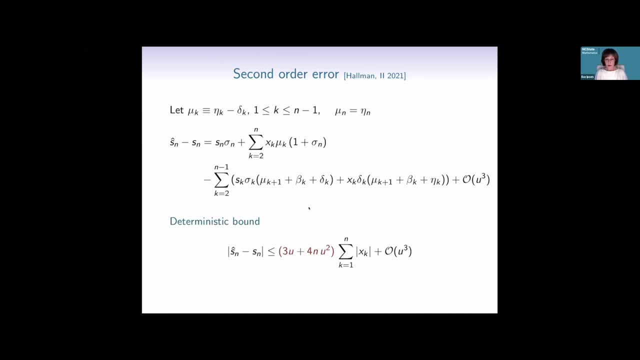 four n times second order unit round off. So, and then we have a probabilistic bound where with high probability, we get here's the first order arrow, and here we have the two norm of x, not the sum of absolute value. So this is a little better here. 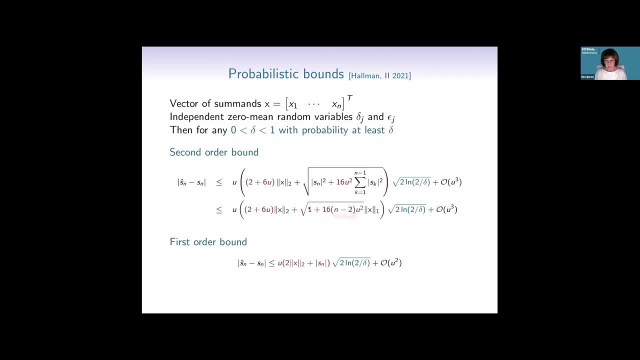 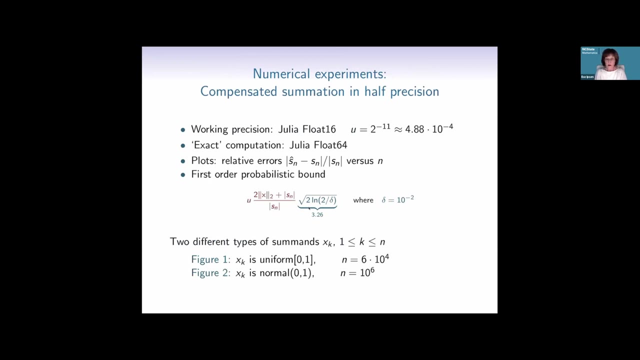 And then here you have a square root over n. So again that that confirms the arrow to to second order now, is proportional to square root of n. So let's do some experiments. So here now I'm going to do things in in half precision. So float 16 in. 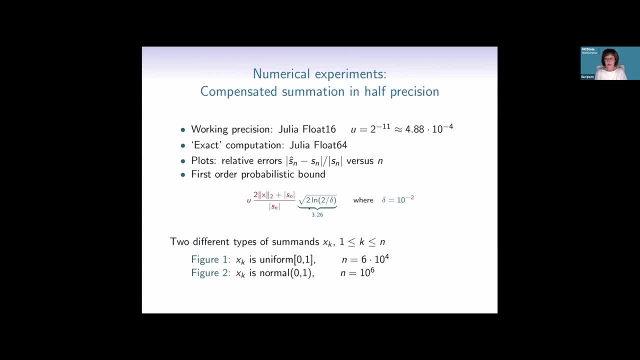 Julia. so they are our unit or unit round off is 10 to the minus four. we are going to do the exact precisions in double precision. we're going to plot the relative arrows versus the number of summons and then our probabilistic bounds. And this 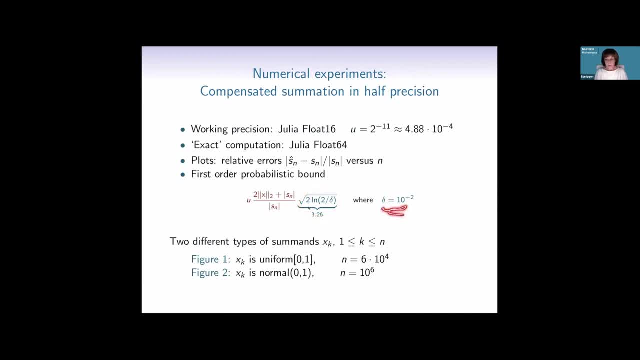 factor we occur here. we are setting the failure probability equal to 10 to the minus two, And then this extraneous factor here comes out to 3.26.. Again, we are looking at our two different types of summons: well conditioned ones and not. 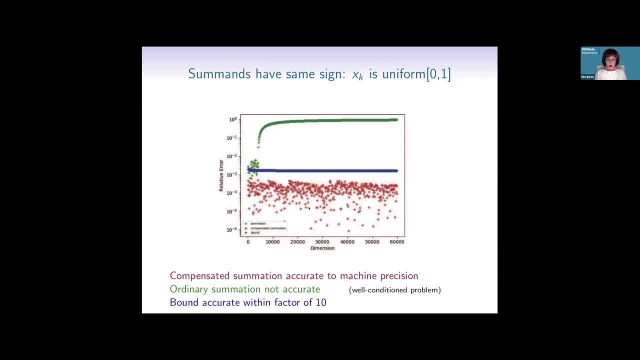 necessarily well conditioned ones. So here's the well conditioned problem, where all the summons have the same sign: Yes, 10 to the minus, 410 to the minus three. So this is what we are entitled to in half precision. So we are. 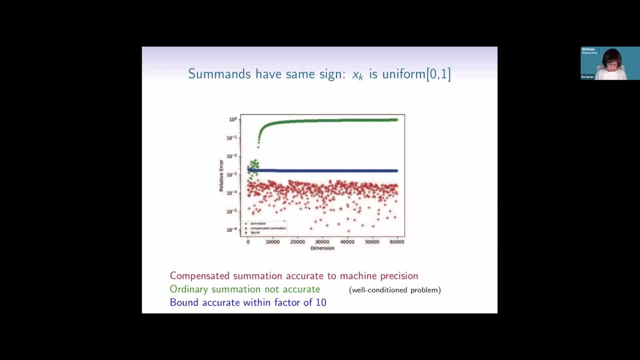 getting machine precision with compensated summation of precision- This is our bound- is pretty good And this is ordinary summation. So here we are, adding only 60,000 numbers, because all the numbers can be in magnitude while they're non-negative right, and the largest number in binary 16 is 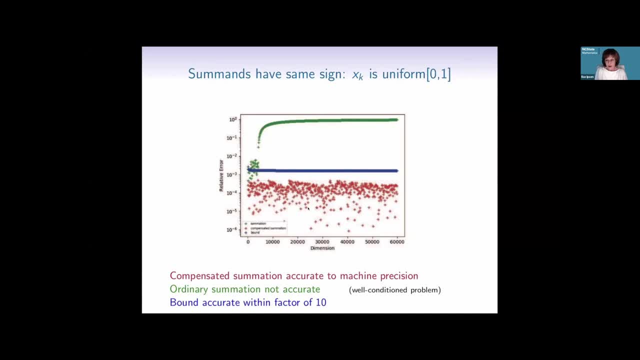 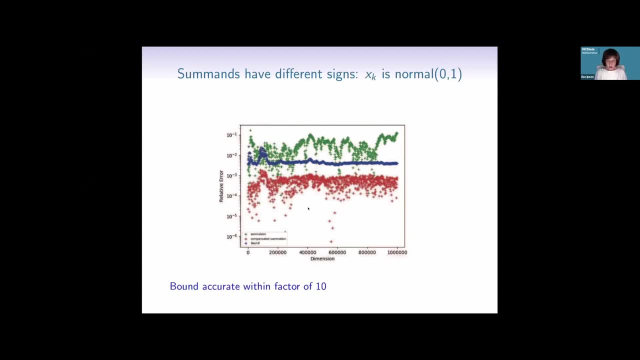 65,504.. So that's as high as we can go, because we don't get cancellation. However, if we allow cancellation, we can add up to 10 to the five numbers here And then you see again: here's 10 to the minus three, 10 to the. 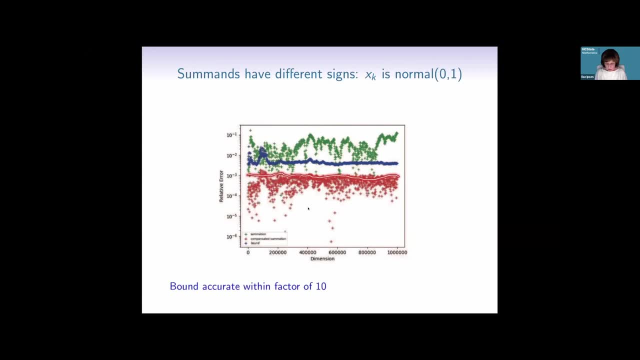 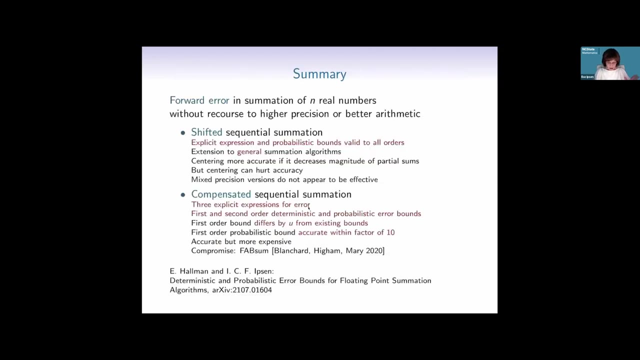 minus four. Again, compensated summation almost gives us unit round off in half, in half precision. Here's our bound, which is pretty good within a factor of 10.. And then here is ordinary summation. Okay, I'm making up for time. Okay, so.